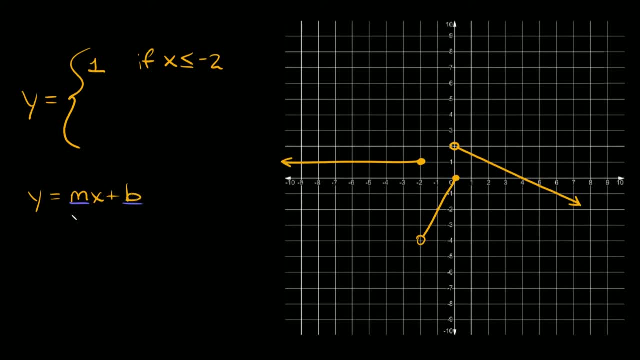 intercept, or in other words where the graph hits the y-axis. okay, So first let's figure out the slope here. So the slope is: let's see, to get from one point to another point on the graph, we have to go up one, two and then over one, right? 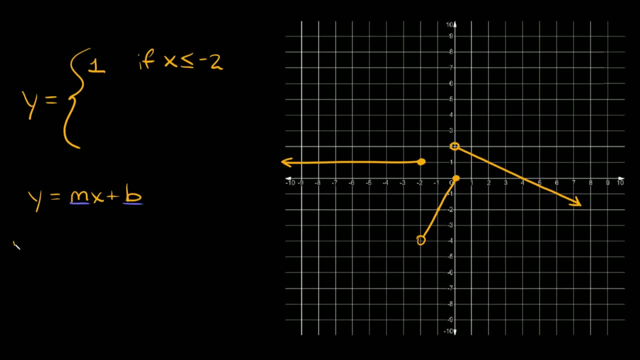 Up two over one. So the slope is equal to rise, the rise over the run. So it's two over one, and two over one is just equal to two, right? So then the slope over here is gonna be equal to two. And then our y-intercept, or in other words again: 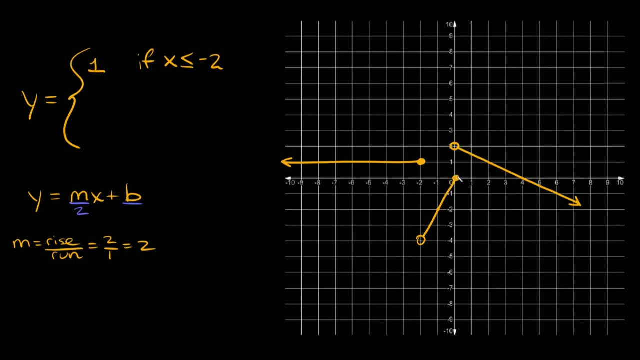 where the line hits the y-axis is right here at the origin, at zero, right? So then we're gonna plug in a zero for b, okay? So then here we're gonna have: y is equal to 2x plus zero, but that doesn't do anything, right? So we can just leave it like this: y is equal to. 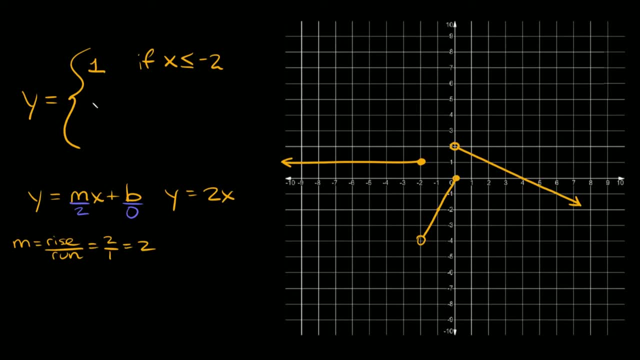 2x. okay, So the equation of this line right here is: y is equal to 2x. right, So y is equal to 2x. Now it's valid, as you can see from negative 2,, right It goes. 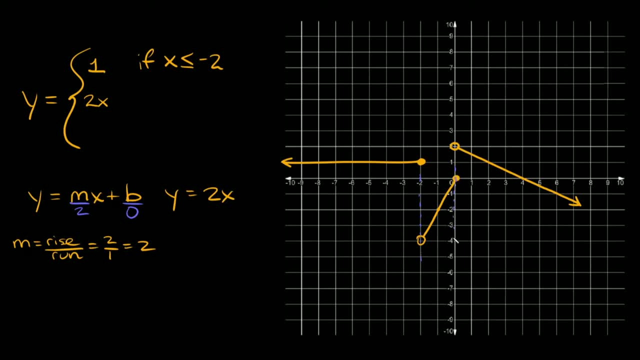 from here all the way to right here at zero, right, So it's good- between this space right here, from negative 2 to 0.. So it's valid when- or I can say, if x is greater than negative 2 and and when it's less than or equal to zero. okay, Here I used a less than symbol. 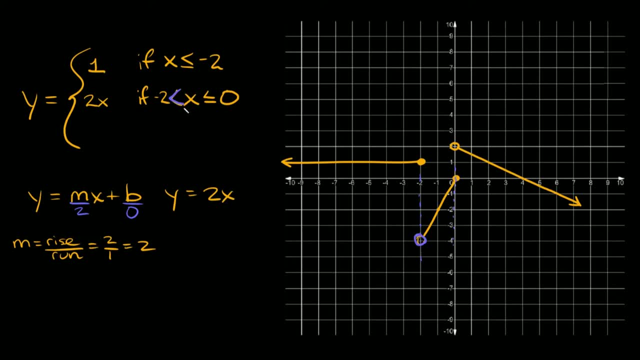 because we have an open circle, right. So we know it's just a less than symbol and here we have a filled in circle. so that's why we used less than or equal to Okay. so again, y is equal to 2x is valid from negative 2 to 0,. okay, And then. 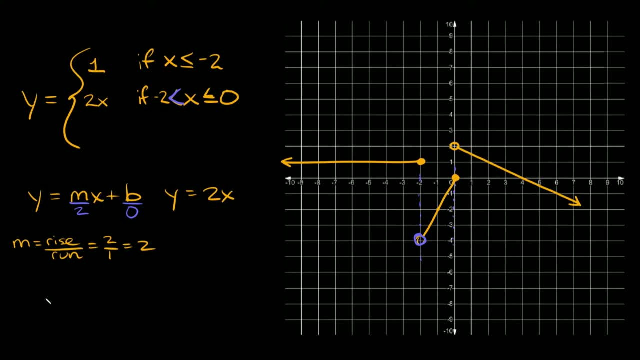 lastly, we just need to find the equation of this line right here. So again we can use: y is equal to mx plus b. so again our slope and our y-intercept right. so our y-intercept in this case is at positive two right, because that's where this line hits the y-axis. it hits it at positive two right here.